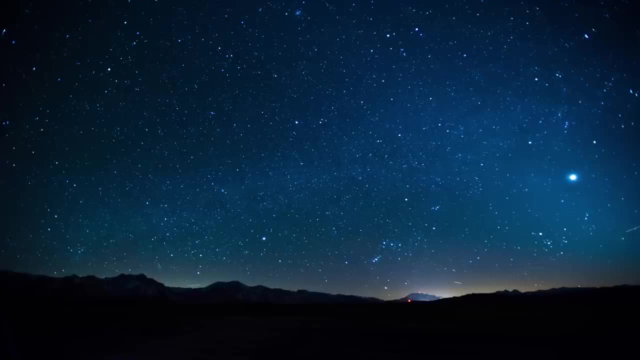 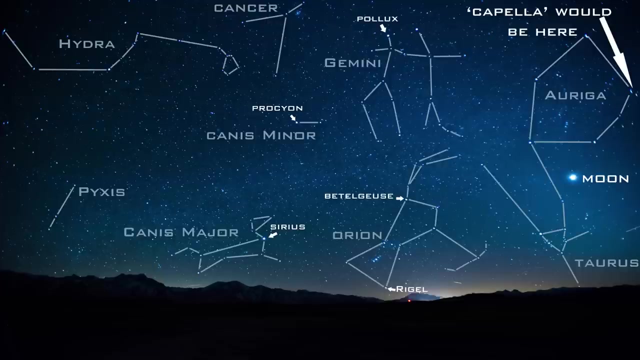 But let's whack up another image of it. It's in there somewhere amongst this celestial orgasm. The belt and the sword are the stars that are immediately striking. So easy to spot, if you can recognise the belt and the sword, Because there is a lot going on in this image, But you just need to know what to look for. But it also gives you an idea of the scale of Orion. It's pretty huge. 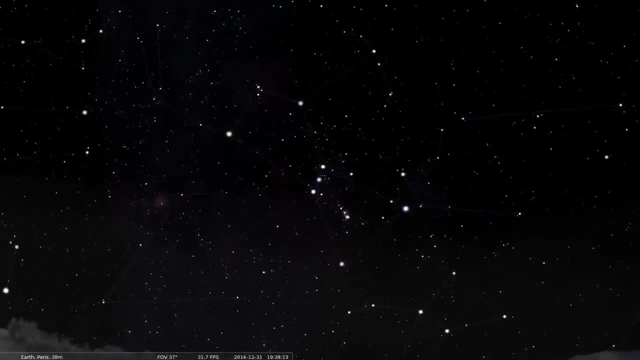 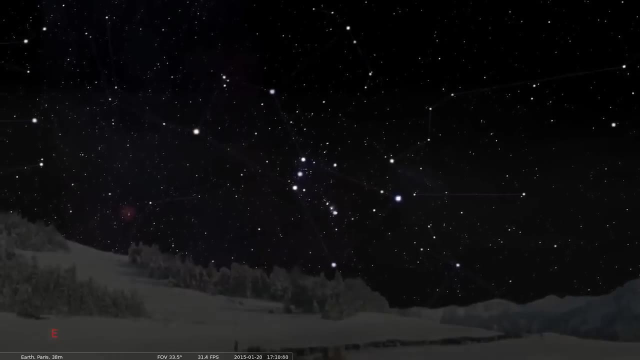 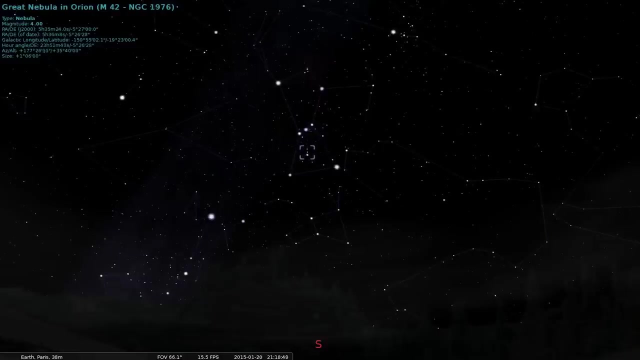 So let's find directions with it. I'll pitch the technique quickly, But then we'll expand on it and further understand it. on a fundamental level, When Orion is tilted to the left and low on the horizon, it is east. When the constellation is upright higher in the sky, it is south. 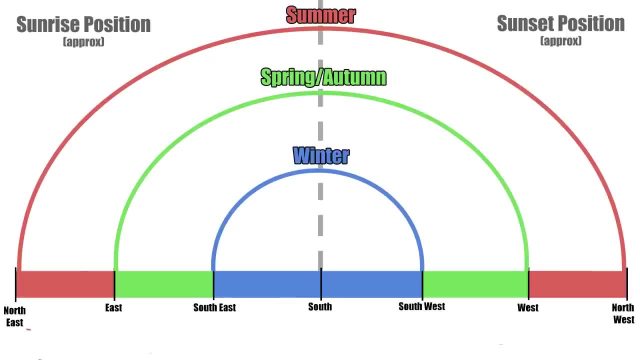 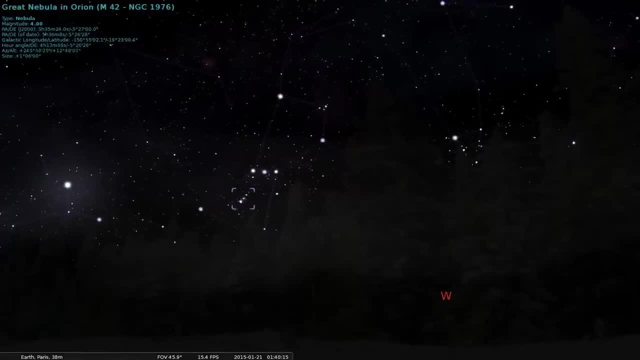 When the constellation is tilted to the right and low on the horizon it is west. Does that ring any bells? Same kind of deal as the fight north with the sun video. Easy right, But we can expand on that, So let's do that And fill in the blanks. 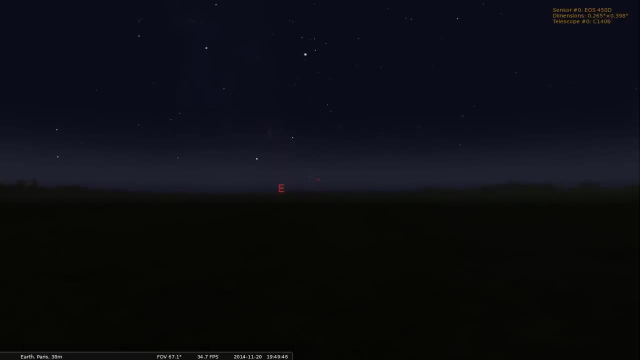 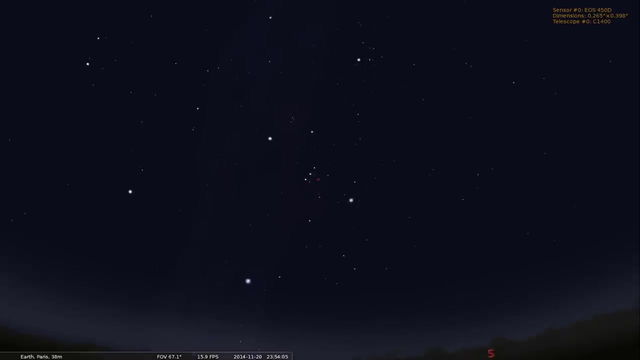 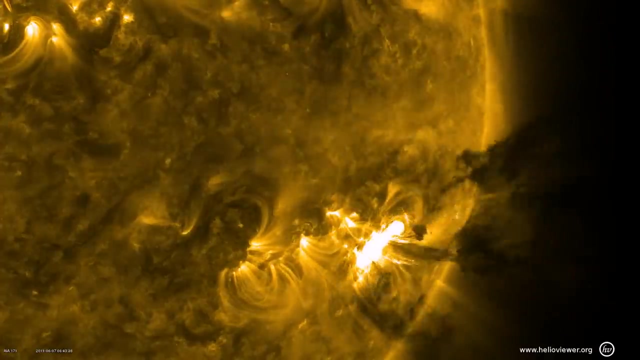 So for a moment let's just track the motion of Orion across our night sky. So it appears in the east, Travels across the southern side of the sky And disappears into the west. Hmm, Does that ring any bells? I can think of another star that follows a similar motion, The goddamn sun. 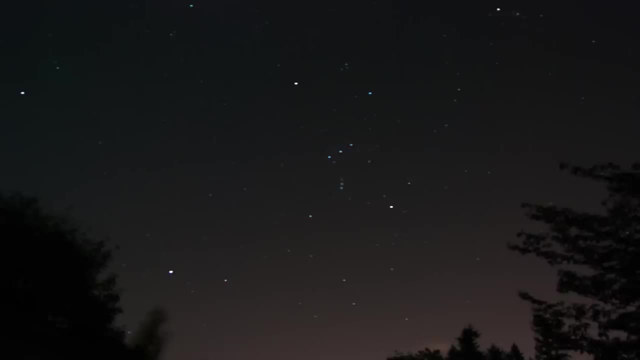 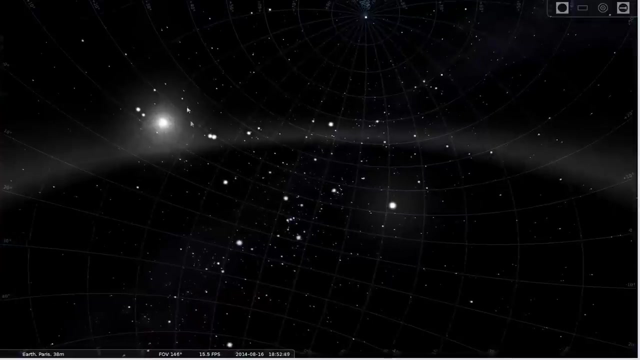 Orion will not be visible in the northern side of the sky. Much like the sun, it sits on the celestial equator. So to put that into perspective, observe the sun, That big old, bright dot, And to the right of it at this current moment in time is Orion. 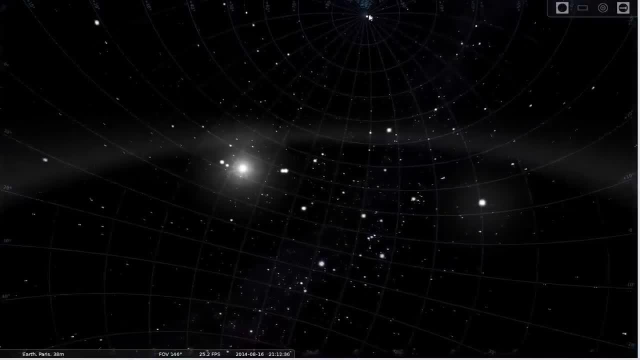 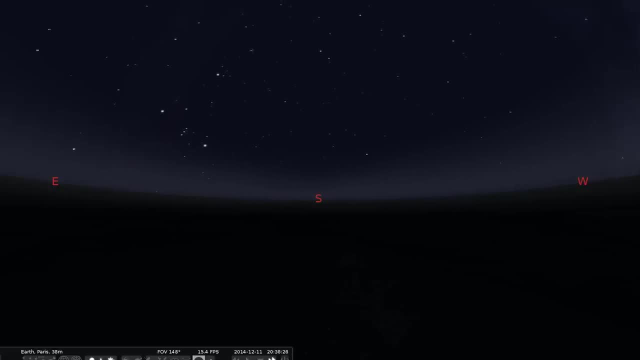 It follows the same equatorial path as the sun, Which is why it's called Orion. Which is why it's called Orion, Which is why it appears in our sky the same way, So fades into the east, travels across the southern side of the sky and eventually fades away into the west. 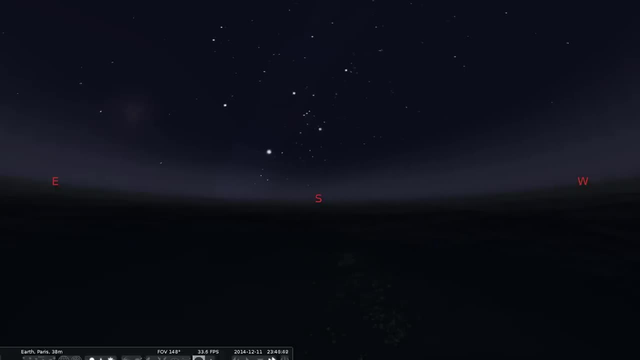 Repeating that for emphasis. So we won't use this constellation to find north directly. Oh no, We will use it to find north indirectly, through using it to find south, east and west. So how? The first thing to take into consideration is its tilt. 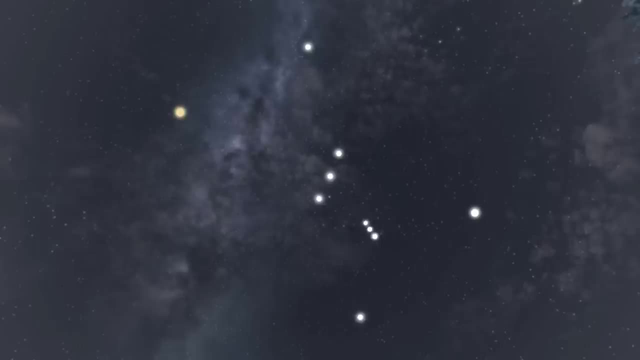 As a general rule, when it's tilted to the left, it's eastward. When it's tilted to the right, it's eastward. When it's upright, it's south. When it's tilted to the right, it's west. 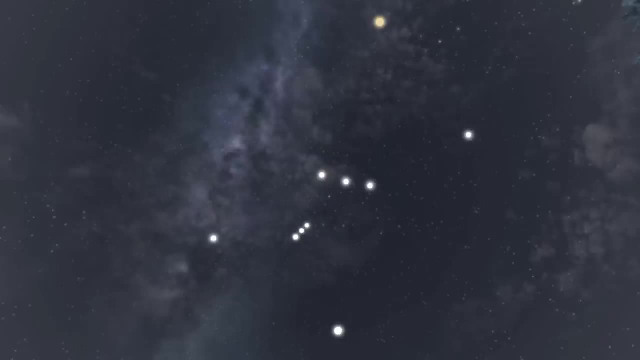 And you can judge the severity of the tilt by looking at the sword When it's at centre stage, completely vertical. Likewise, on the horizon it's pretty diagonal, Because the constellation is a bit wonky, admittedly, But the sword is there as a guide if you need it. 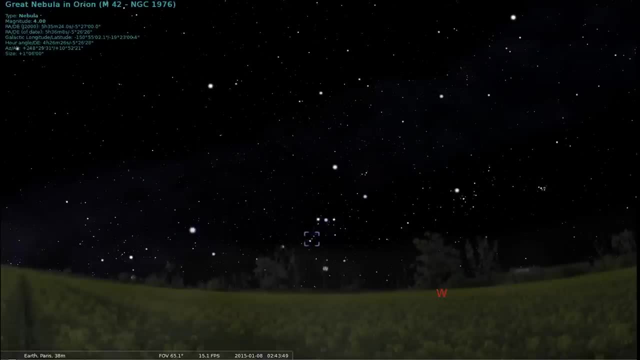 The second thing to take into consideration is how close the constellation is to the horizon. Obviously, if it's low on the horizon and tilted, then it's either going to be east or west right, As it's higher in the sky and less severely tilted. 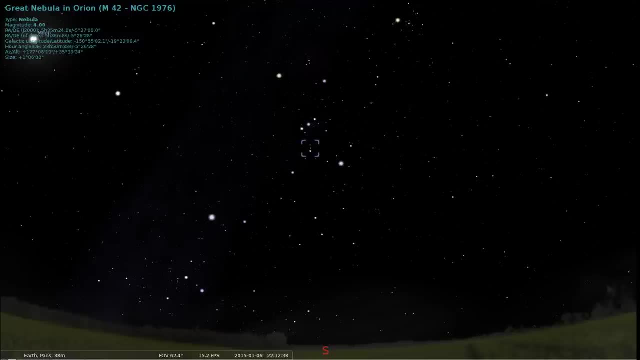 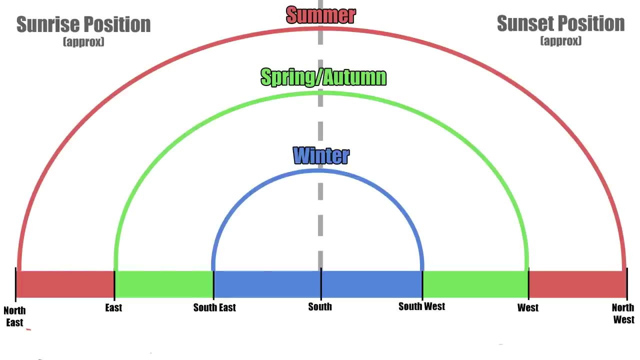 south-east and south-west At its highest point in the sky, when it's upright south. So if you think back with the find north, with the sun video, same kind of deal there. So let's play with some examples. 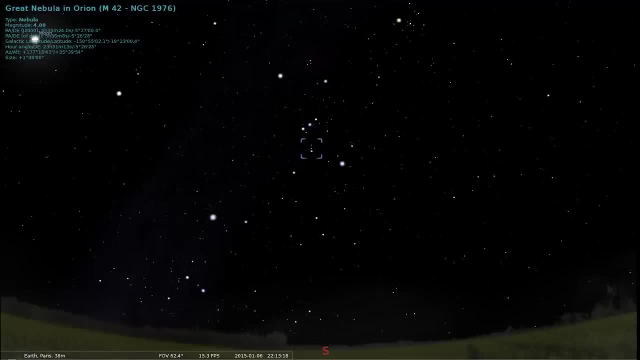 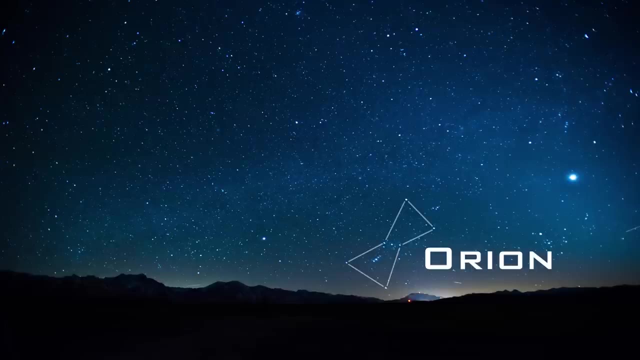 I'm going to give you an image of Orion and you have to work out the direction you're facing, based on the tilt of Orion. So here's Orion laying very low, close to the horizon. So, knowing what we know now, we can conclude that we 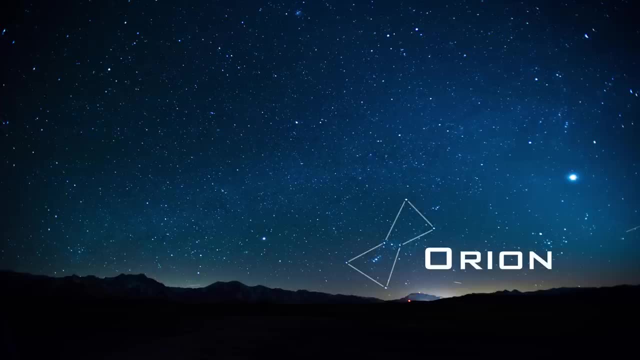 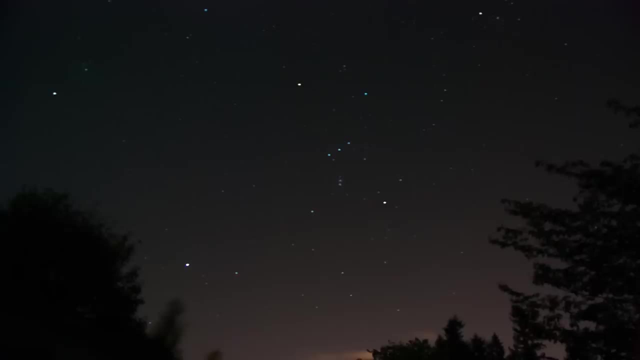 or at least a photographer that took this image- is facing west, And you'd be right about that. Now, how about this one? Well, we can clearly see that it's upright, So we must be facing south at this current moment in time. 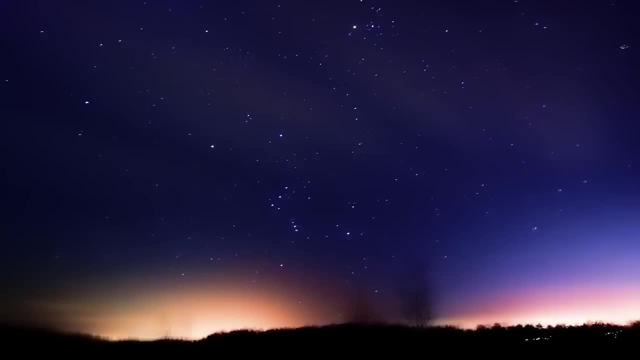 You'd be right. So how about this one? Well, if we analyse it, it's tilted to the left, but it's not laying very low on the horizon. It has travelled upwards a fair amount, So it's not east. 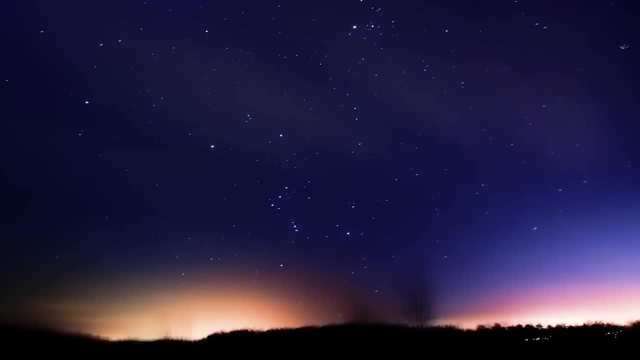 and it's not completely vertical, so it's not south. The middle ground south-east, And you'd be right about that. See how easy this is. That's the skill in a nutshell, GG. So south, south-west, west, easy. 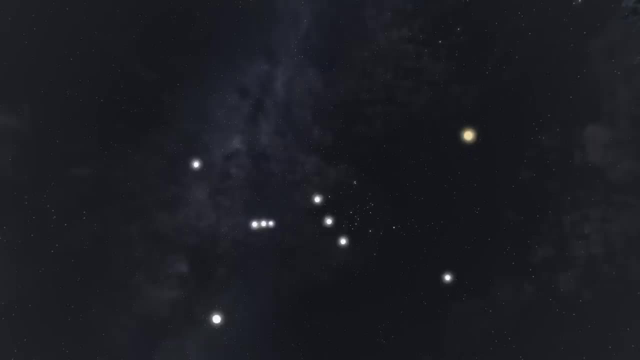 But what if you observed Orion like this? You probably would say west, and you'd be right if you were at the equator, very low in the northern hemisphere. Why? Because as we head closer to the equator, Orion travels higher across the equator. 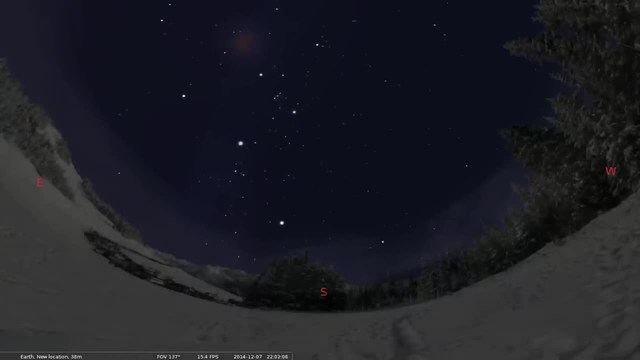 across the centre of the sky So you can observe a much fuller range of motion. It goes vertical at south to completely horizontal, pretty much at the horizon. So for low latitudes you have to take this into consideration. Upright south, tilted south-west, horizontal west. 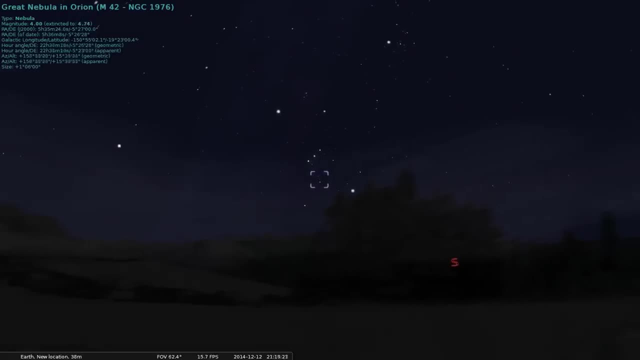 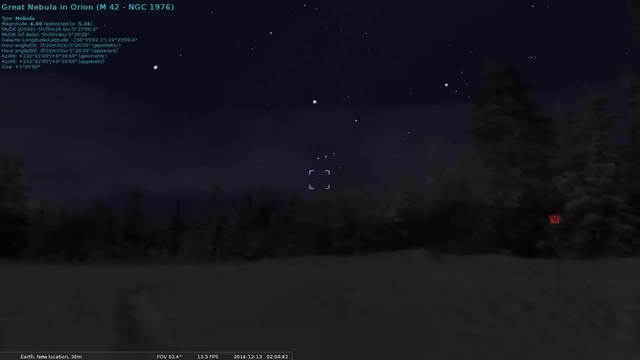 Likewise at the opposite end of the hemisphere, talking boreal or arctic regions, you observe a much shorter range of motion, so it doesn't tilt a whole lot. But the whole tilt game isn't really the deal breaker with this skill. 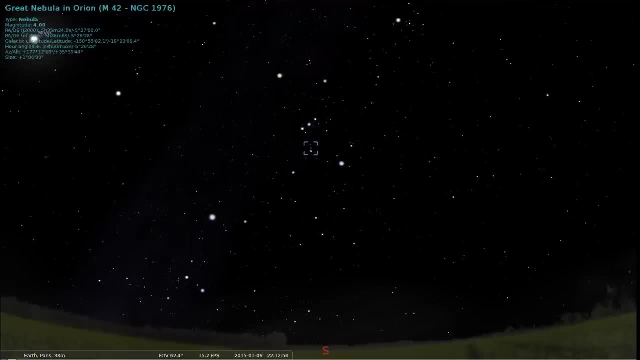 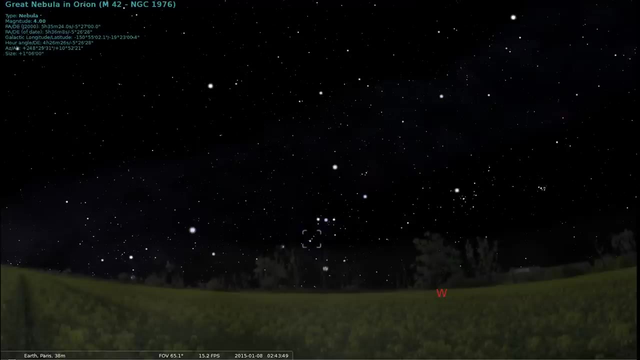 It's always south. when it's upright and vertical. that is a constant. When it's low on the horizons, it's either east or west. that is always true as well. The degree of tilt changes in extremes of latitude, so that's where you either have to do the work. 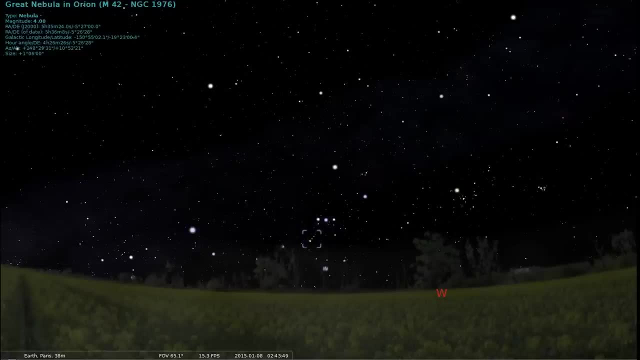 and figure things out for yourself, for your own specific latitude, or if you're lazy, then you don't really need to concern yourself too much with the whole tilt game. Just focus on how close it is to the horizon. You can work out whether it's south-east or south-west. 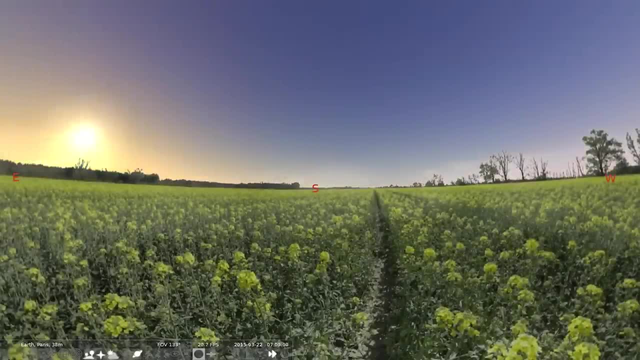 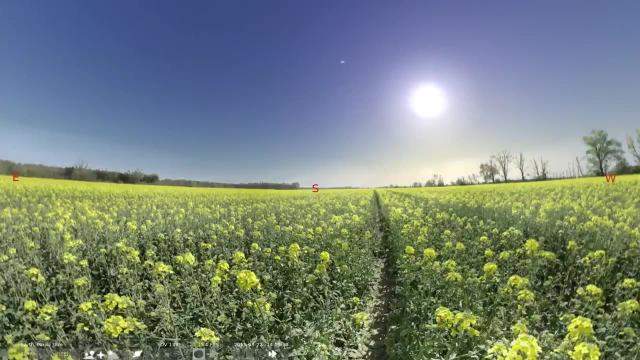 based on how far it is from the horizon. Much like a sunrise. you know the sunrise in the east as a general rule and sets in the west. think of Orion as a night-time sun mimic. That's basically how this works. So now, if we look at this image, 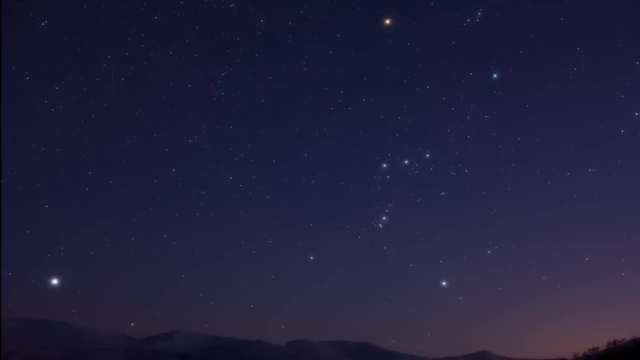 as you can see, it's pretty close to the horizon, yet it's almost vertical. From this one can conclude that this photograph was taken at a very high latitude in the northern hemisphere, probably the top of Norway or somewhere like Iceland as an example. 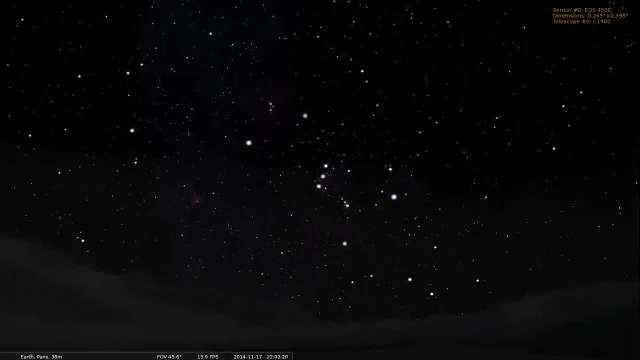 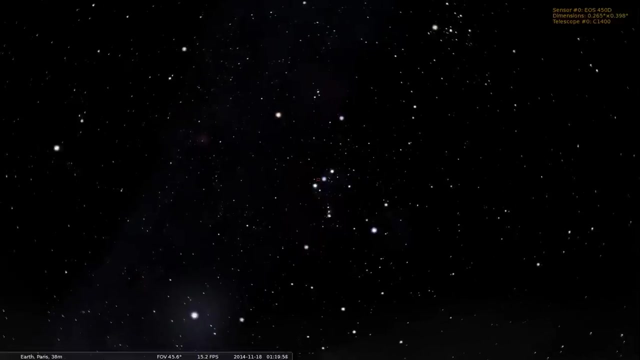 So that is Orion in a nutshell. We know how it travels across the sky in high, medium and low latitudes in the northern hemisphere. We know why it travels across the sky with a similar motion to the sun, and we know how to analyse it to find directions. 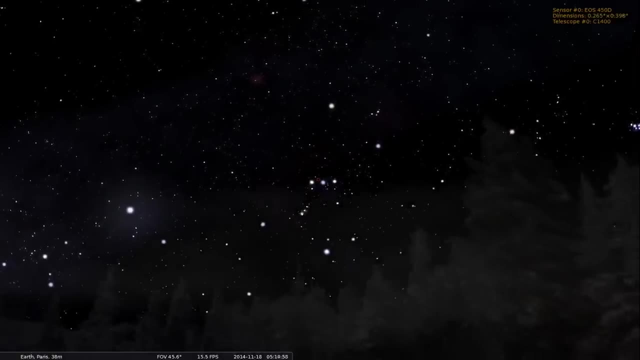 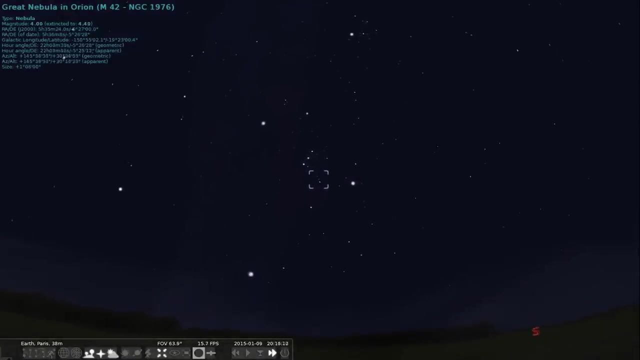 What else can we talk about? Well, let's talk about the ever-changing window for observation. Orion is a seasonal constellation, meaning it will only be visible or partially visible during certain seasons. It's regarded as a winter constellation because during the winter, 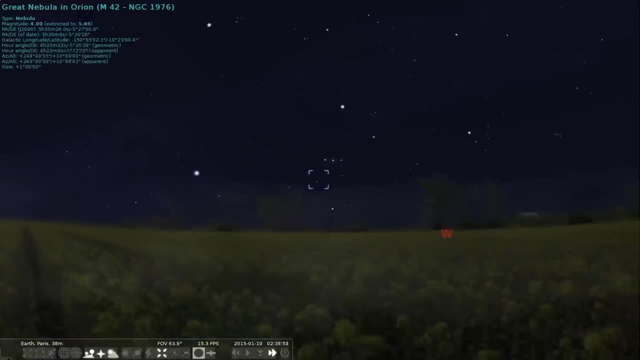 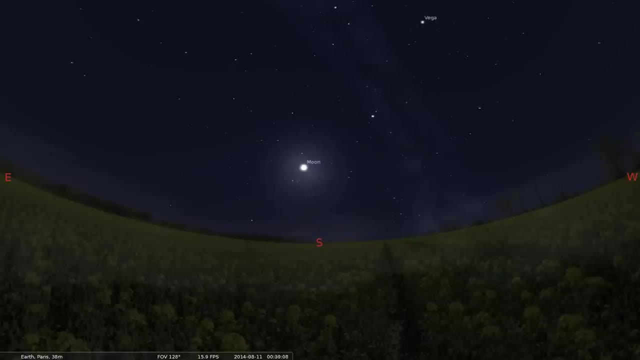 it completes the full visible cycle from east through south to west. As winter transitions into spring it only becomes visible in the south and sets in the west. From mid-spring through to summer it's not visible at all. The constellation becomes visible again in the late autumn. 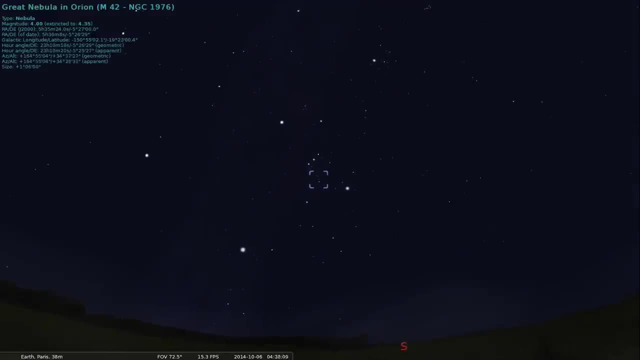 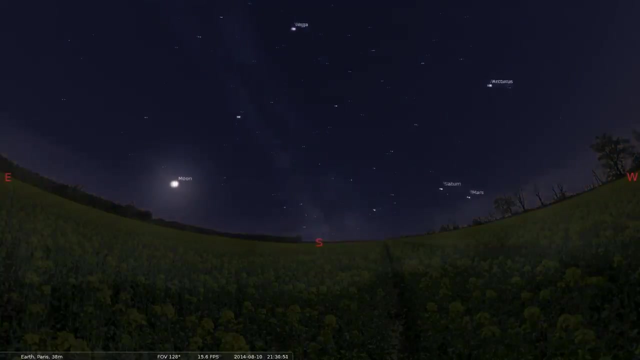 appearing in the east and disappearing into the south until winter comes along and everything's hunky-dory again. So if you go outside tonight, you won't see it. You've got to wait a while before you can revel In the majesticness of Orion. So that's curious. What is the reason behind it only being partially visible during certain seasons? It's to do with our position around the sun during those seasons. A short answer: In the winter, shorter days, longer nights, so we can observe more of Orion. 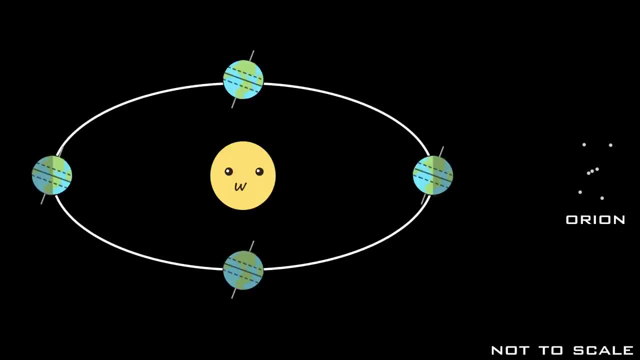 In the summer: longer days, shorter nights. So yeah, but that's not really the real reason at all. The long answer? Well, we'd have to get talking about perspective, in accordance to our position around the sun During the four seasons. 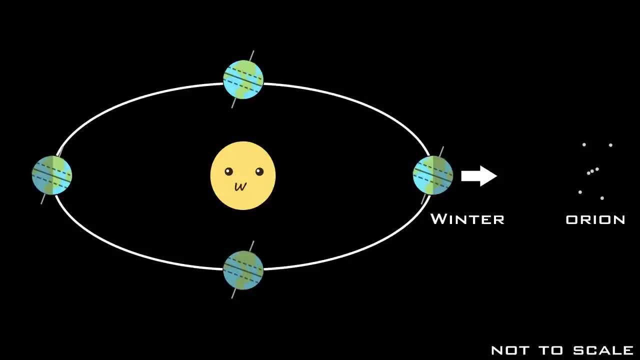 As we're over here in the winter, tilted away from the sun, we have a full 12-hour night time, to simplify it, pretty much facing directly towards Orion, So we can see its glorious full range of motion across our night time sky. 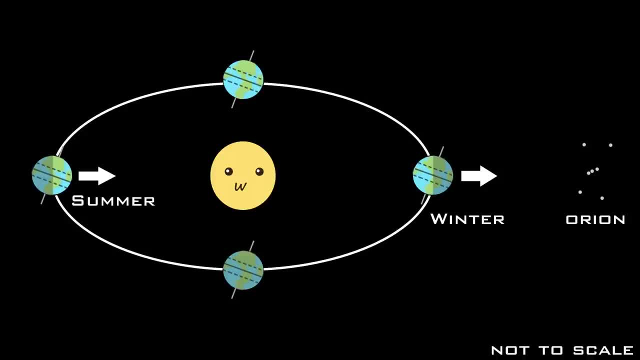 As we're in the summer over here. basically, the sun is in the way. Well, it's not really in the way. The sun isn't so massive that it blocks our view of star systems that are 1,300 light years away. 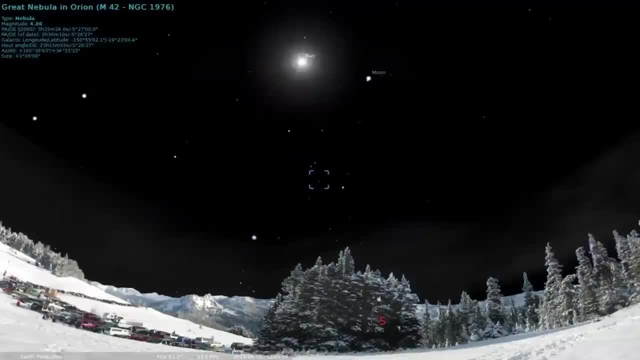 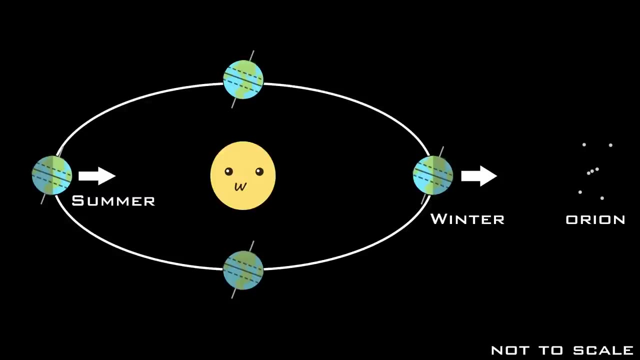 We would see Orion during the day, but you know, the sun's out, so Rayleigh scattering prevents us from seeing out of our atmosphere. As night time rolls around, we're facing in the opposite direction, So we observe a new set of stars. 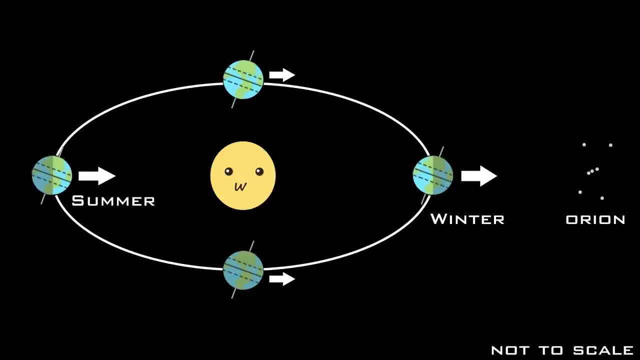 Orion is nowhere to be seen. As we're in spring and autumn, we can see half of Orion's full motion, before Rayleigh scattering, prematurely comes back around as night transitions into day. Right, Okay, so there you go, Finding directions with Orion. 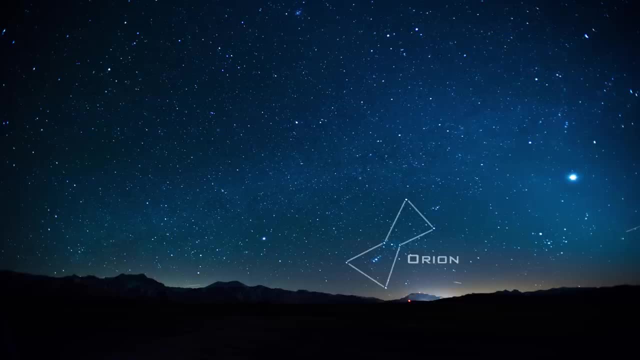 plus a whole lot more Orion-related stuff. One more thing before I go though. A bonus pro tip: If you follow the belt of Orion, create an imaginary line that extends outwards to your left, you'll bump into a very bright star. 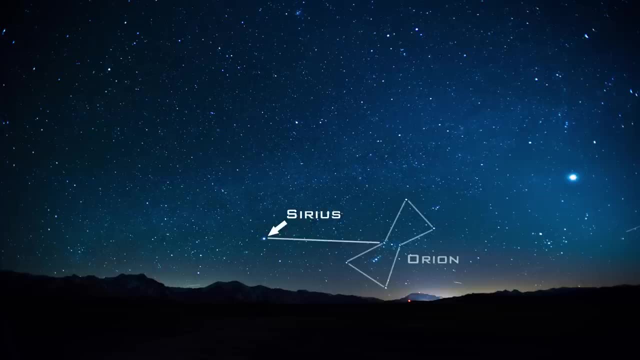 And that star is called Sirius, one of the brightest stars in our night sky. So that's easy to remember, right? It belongs to the constellation of Canis Major, which looks a bit like a dog, right, A little bit, Has a very bright, shiny star on it. 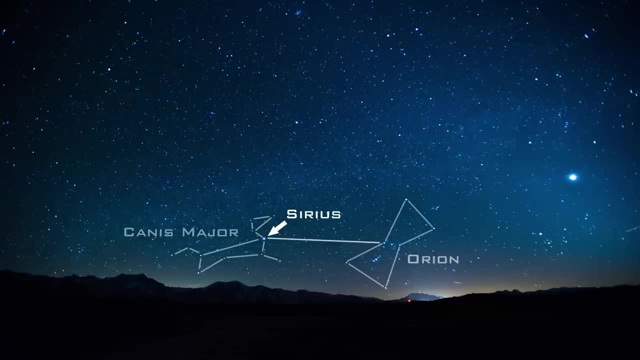 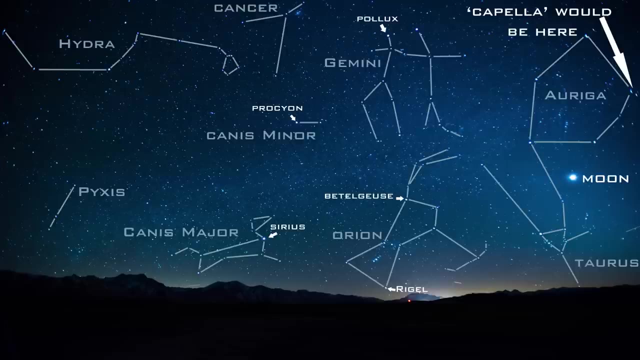 It's Collar. Canis is actually the genus for wolves, jackals, dogs, coyotes, canine. You dig it Cool. So that's that, Just for the sake of knowing things. Canis Major and Sirius aren't used for as navigational aids. but I figured I'd mention it so you could add another celestial knowledge notch to your bedpost: Orion, Sirius and Canis Major. 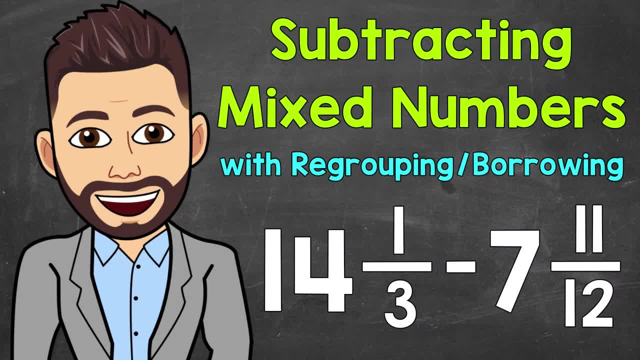 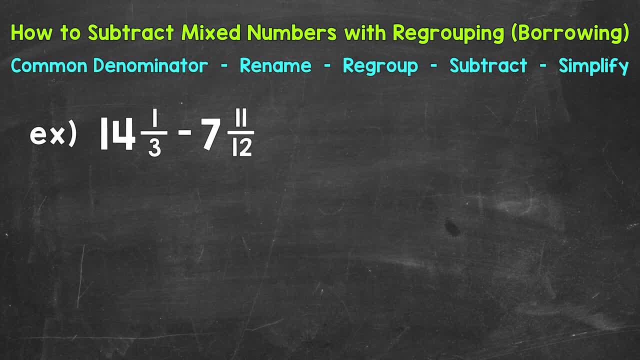 Welcome to Math with Mr J. In this video, I'm going to cover how to subtract mixed numbers with regrouping, also referred to as borrowing. Let's jump into our example where we have 14 and 1 third minus 7 and 11 twelfths.